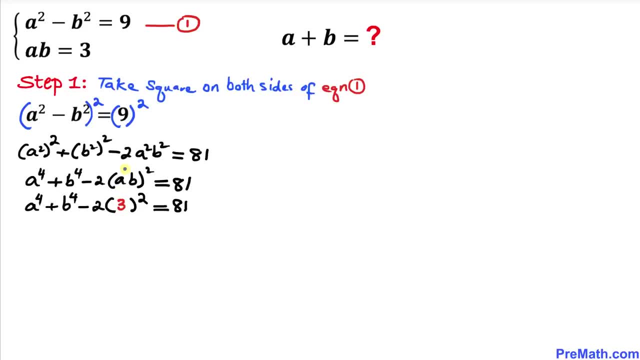 by three. and here, in the next step, I replace this a times b by simply three, and the rest is same. and now let's focus on this part: two times three, power two. and here I have copied it down and we are going to take care of the exponent first. So two times three, square is going to 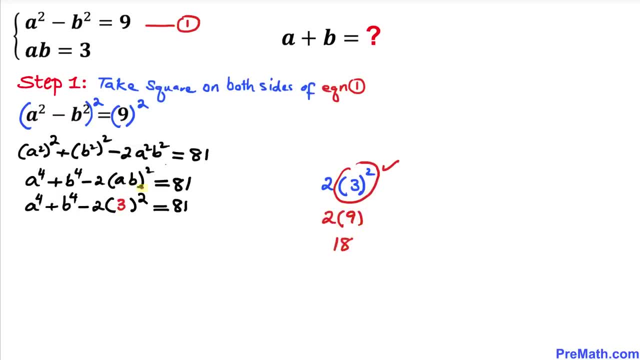 become nine. Two times nine is eighteen, so therefore I am going to replace this whole thing by eighteen. So therefore our equation is simply going to become: a power four plus b power four minus eighteen equals to eighty one. And now let's go ahead and add eighteen on both sides. This is gone. so we simply ended up with: 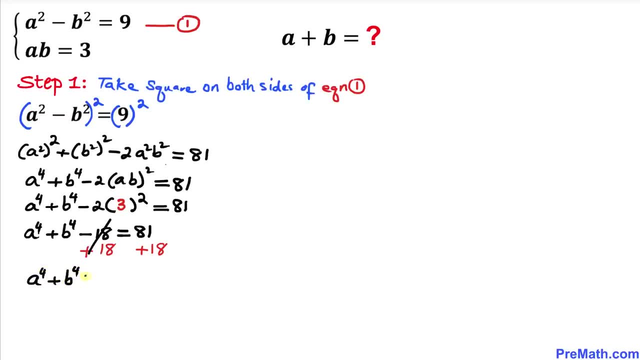 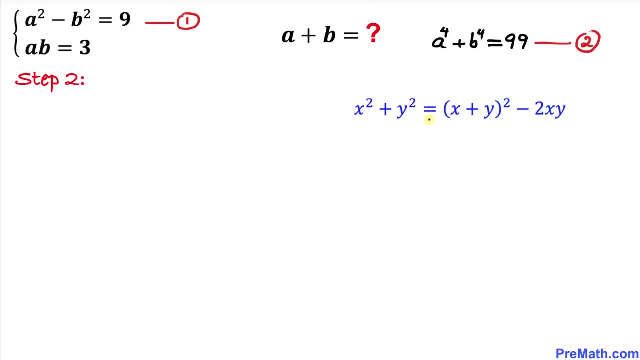 a power four plus b power four equals to ninety nine. Call this as an equation number two. and here is our next step. Let's recall this Identity: x square plus y square could be written as x plus y, whole square minus 2 times xy. 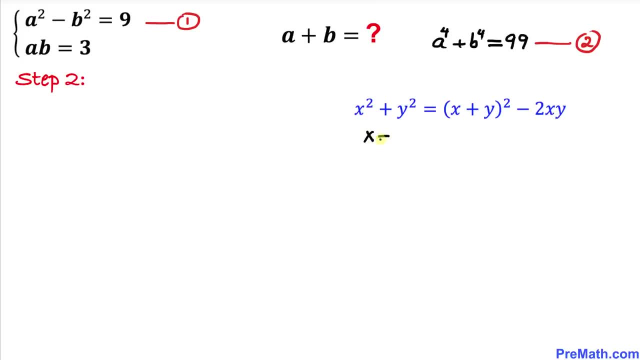 If I let x equal to a square and let y equal to b square, then this identity is going to simply become a square and then a whole square plus b square. whole square equal to a square plus b square, and then a whole square minus 2 times a square times b square. 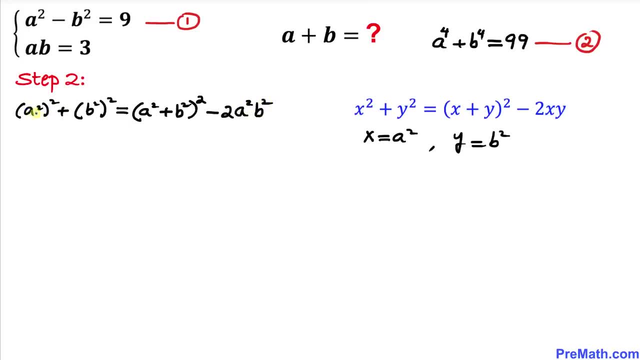 And now let's go ahead and apply the rules of exponents. So on this side, a square and power 2 is going to become a power 4. likewise, plus b, power 4 equals to. I'm going to leave this one as it is. 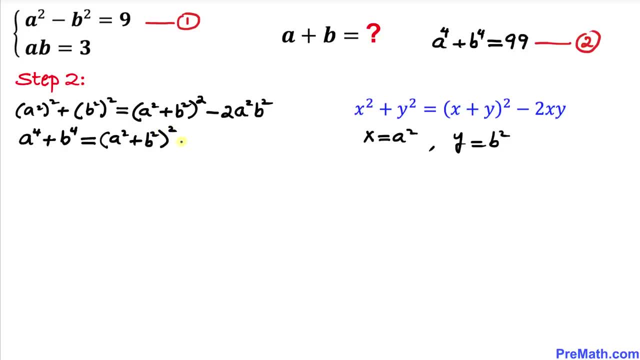 a square plus b square, whole square minus 2 times a square. b square could be written as a, b, then whole square, And now we know that this a power 4 plus b power 4 equals to 19.. So I'm going to replace this one by 99 and likewise this a times b. 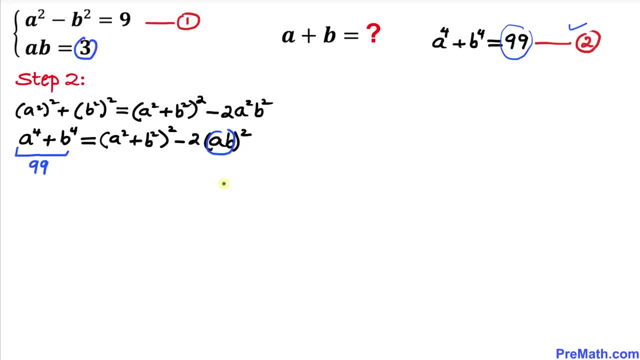 I'm going to replace it by 3.. So we can write this one as 99 equal to a square plus b square, whole square minus 2 times 3 whole square. And now let's focus on this part. I have replaced it over here, and this could be simplified to 18.. 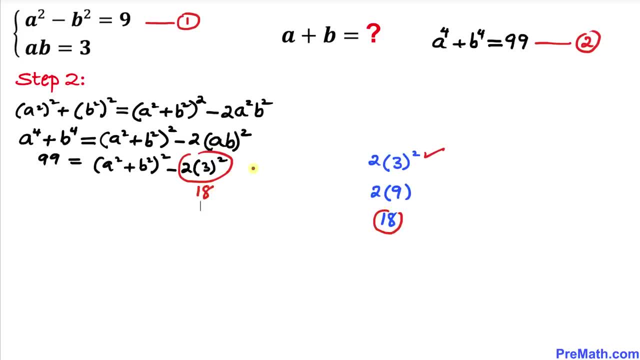 So, therefore, I'm going to replace this one by 18.. And here, in this next step, I have replaced this part by 18 and the rest is same. Now let's go ahead and add 18 on both sides. This one is gone. 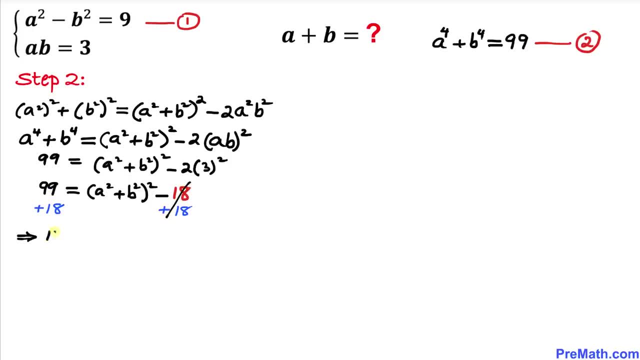 So we ended up on the left hand side. that is going to give us 117, equal to a square plus b square- Whole square. or we can write this equation the other way around. Now let's go ahead and take the square root on both sides of this equation. 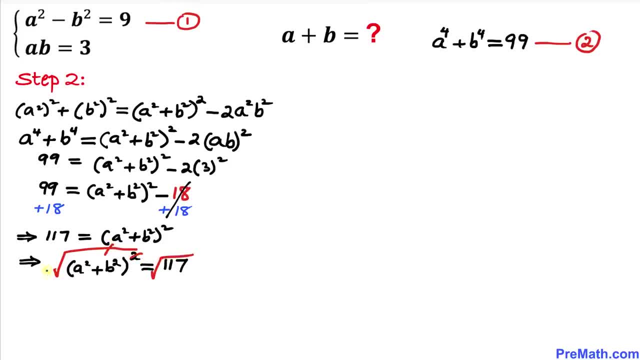 This square and square root is gone, So we ended up with simply a square plus b. square equals to positive or negative, And the square root of 117 could be simplified as 3 times b And the square root of 13, as you can see over here. 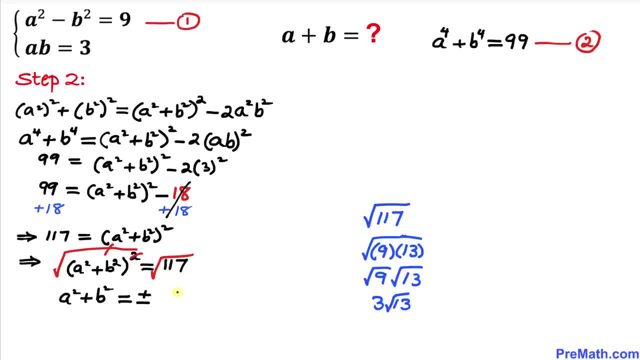 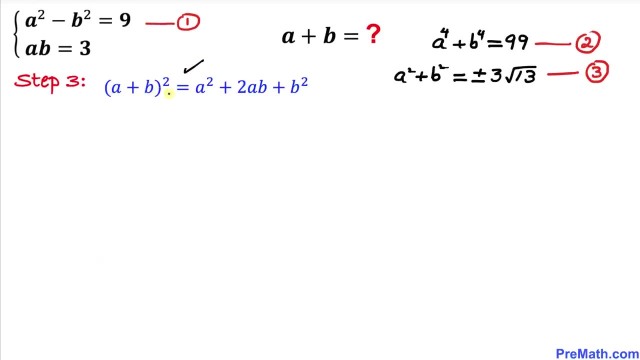 So this could be written as positive or negative: 3 times square root of 13.. Let me go ahead and call this as an equation number three. And here's our next step. Let's recall this famous identity: a plus b square equals to a square plus 2ab plus b square. 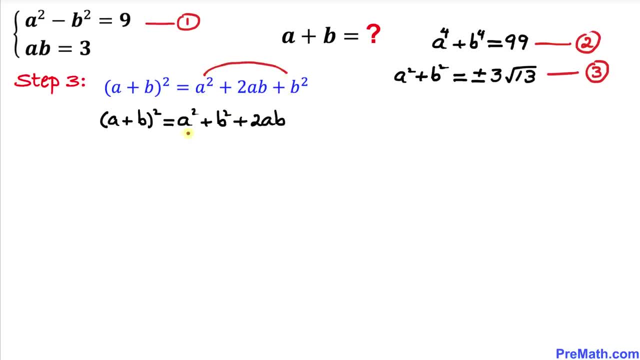 And here, in this next step, I have rearranged these a square and b square over here, And now we can see that a square plus b square is positive or negative. three times square root of 13. from this equation three, And our a times b is three. 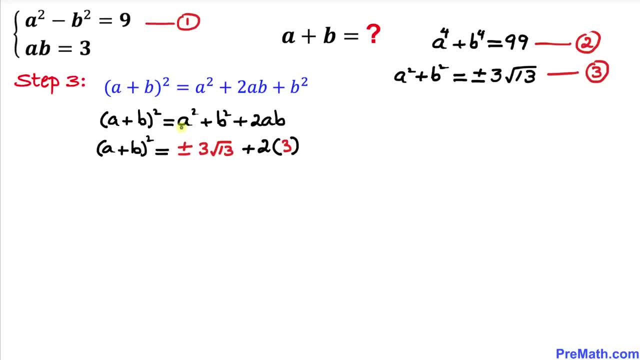 So I'm going to replace this one by three. And here, in this next step, I have replaced this a square plus b square by this positive or negative three times square root of 13.. And here I have replaced is a, b by 3, so our this equation is simply is going to become a plus b whole square. let me go. 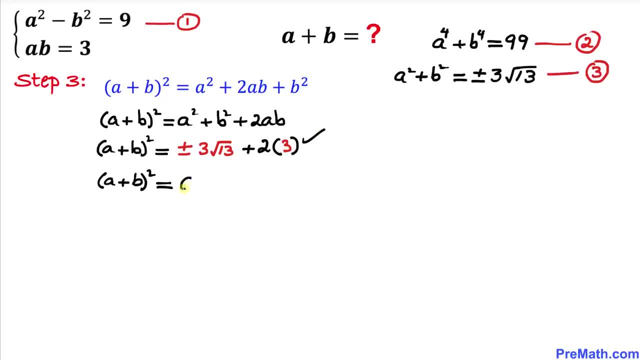 ahead and take care of this one first. 2 times 3 is 6, and then I'm going to write down positive or negative 3 times square root of 13. we can write this one as a plus b, whole square equal to 6 plus 3 times square root of 13, and the other value is going to be a plus. 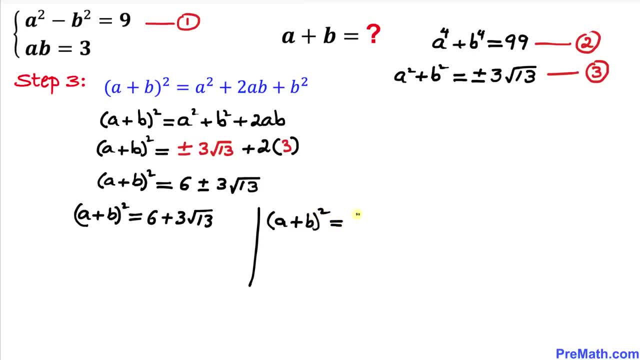 b whole square equal to 6 minus 3 times square root of 13, and here we can see that we have a positive sign and negative sign as well. now we can see that this value is greater than 0 and if we look at this value, this is less than zero. but then we know that this a plus b whole 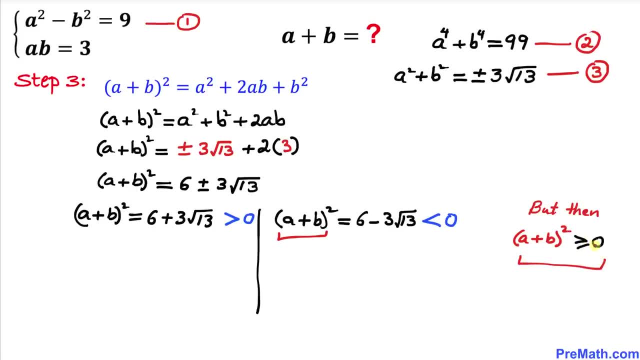 square is always greater than or equal to 0, and here we have this: less than zero. so therefore, this is a false statement. therefore, we are going to reject this scenario and we are going to accept this one. and now let's go ahead and take the square root of 12 plus b, whole square plus 2. of 0 and the value of 12 here is negative, so this is a minus sign and negative sign, which is a positive sign, so this is also negative. so if we try to get an example here, the first equation, we have a substitution circle. so we are going to write down the situations. 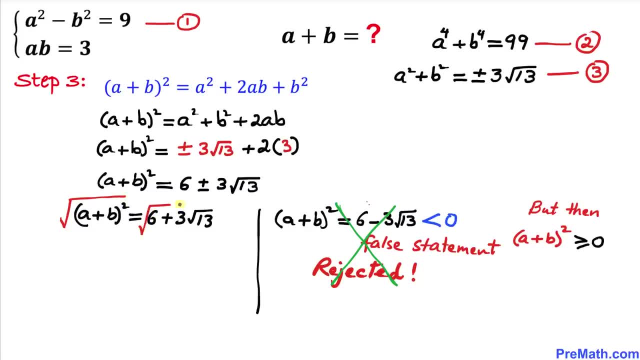 on both side- on this one and on this side as well- and here this square and square root, they undo each other. so we simply got a plus b turns out to be positive or negative, square root of 6 plus 3 times square root of 13, and that is the value that we were looking for. so that's our a. 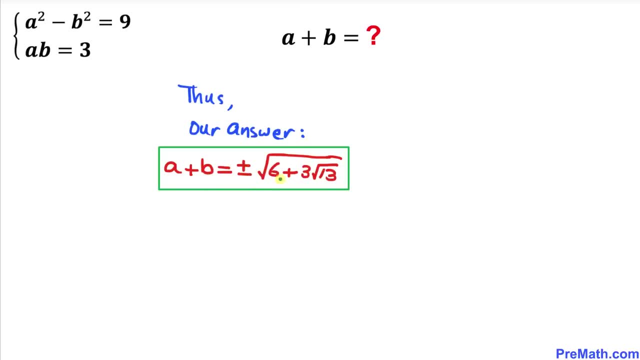 plus b value turns out to be a positive or negative square root of 6 plus 3 times square root of 13, and that's our final answer. thanks for watching and please don't forget to subscribe to my channel for more exciting videos. bye.